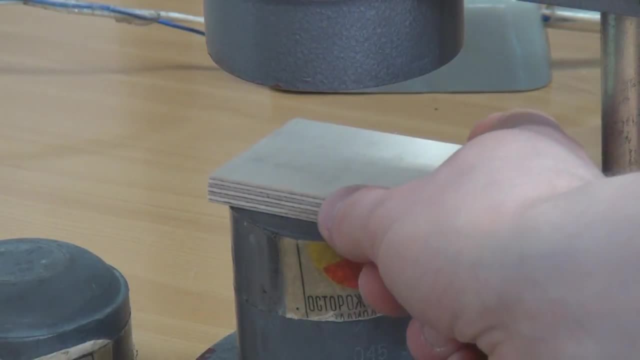 Now it's time to measure the radiation directly emitted from the exposed radioactive material, And the result is 567 counts, which is seven times larger than the natural background radiation. In order to see how efficiently wood blocks the data, Let's take a look at what would be a difference into the radiation of wood, aluminum, steel and human in the field. 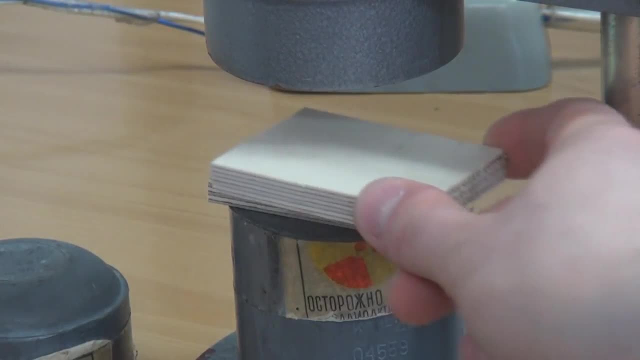 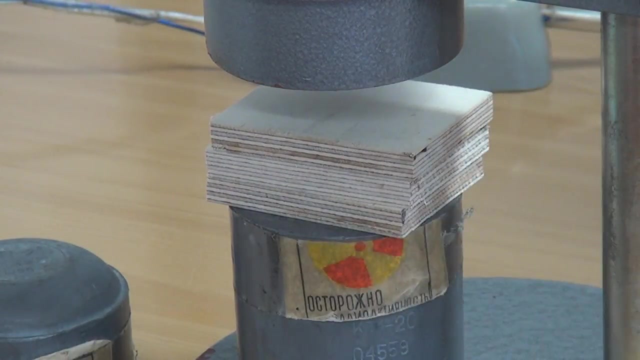 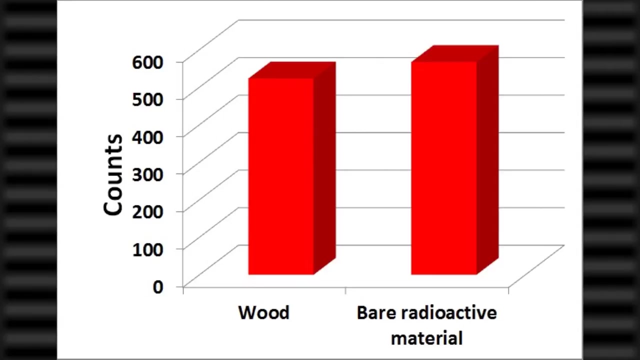 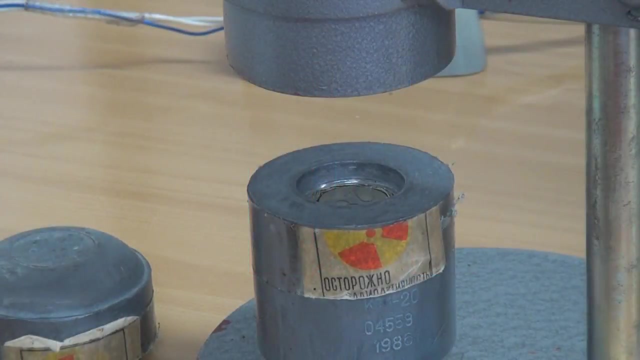 dangerous gamma rays. we placed a thick layer of wood between the radiation source and the geiger counter. 523 counts within 100 seconds is pretty close to the amount measured with pair radioactive substrate and clearly shows that wood is an extremely bad material for protecting yourself from nuclear radiation. next we decided to test aluminum as astronauts spend. 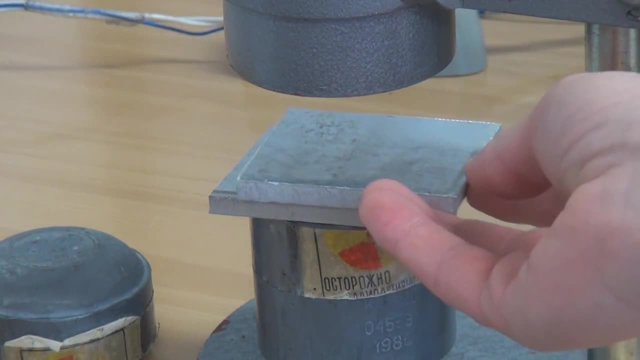 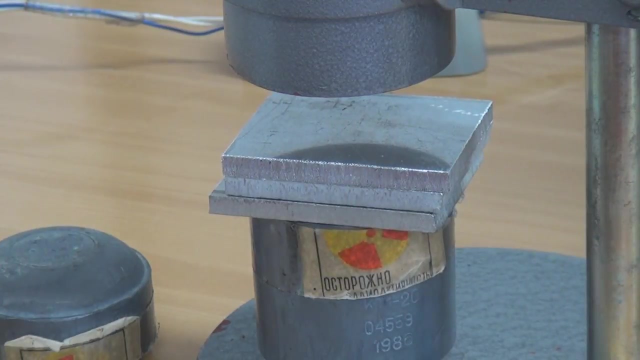 a lot of time in space, and the spaceship has to be prepared from light materials such as aluminum alloys. therefore, we used 24 millimeters of aluminum, as that's how thick the spaceship's walls are. after 100 seconds of measuring, we see 450 counts, which means 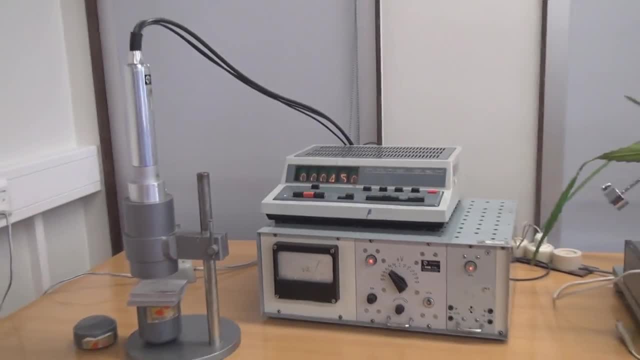 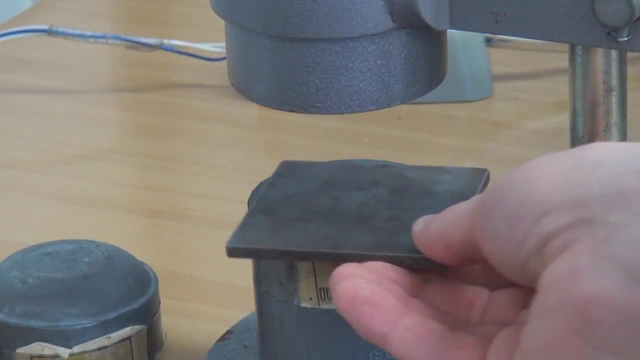 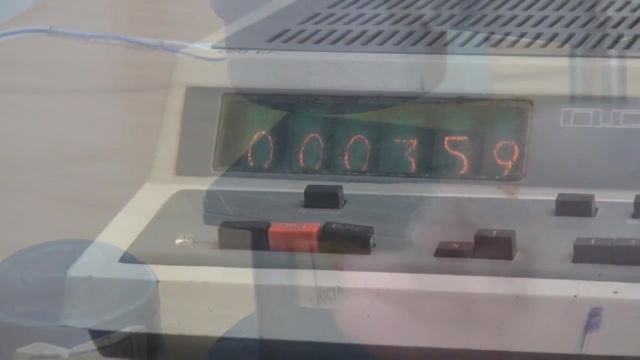 that spaceship walls made of aluminum hardly protect the astronauts from gamma rays. one of the most common materials in the world is steel, and therefore we decided to test 18 millimeters of steel for radiation shielding, as this thickness is common in mobile infantry military vehicles. steel with this thickness can stop a bullet and apparently it also significantly. 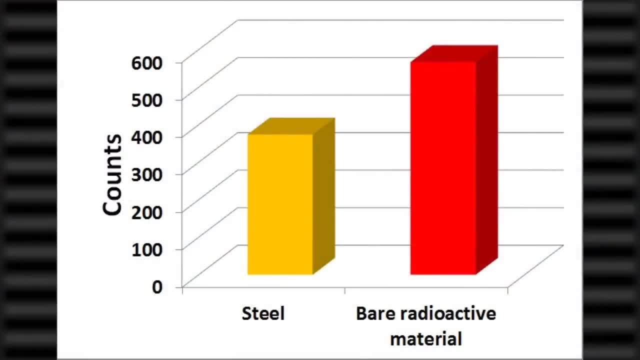 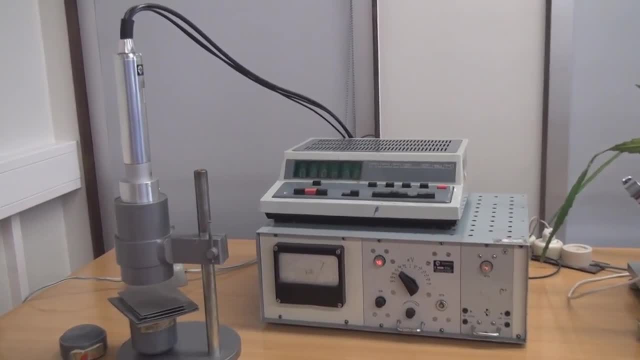 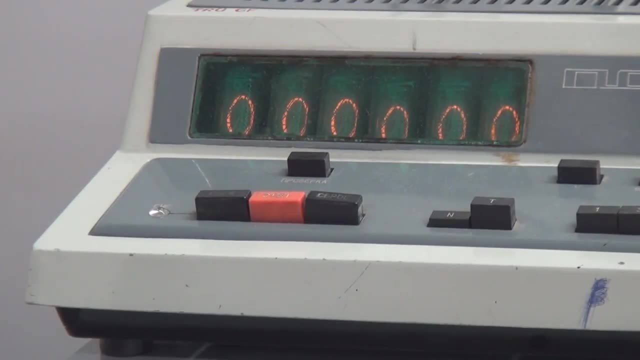 but not completely blocks nuclear gamma radiation, as the penetration of the radiation strongly depends on the atomic number of the material. we also decided to test tungsten that has a high atomic number and extremely high melting temperature. although tungsten layer was only 5 millimeters thin, it 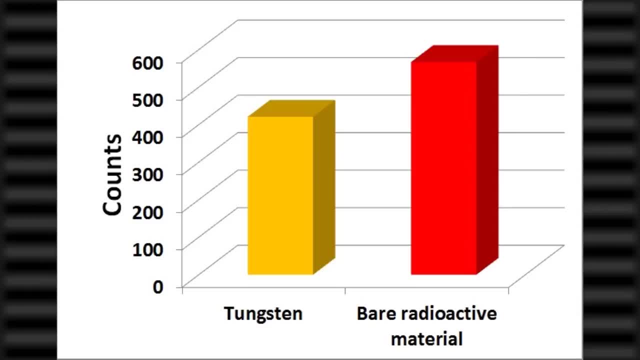 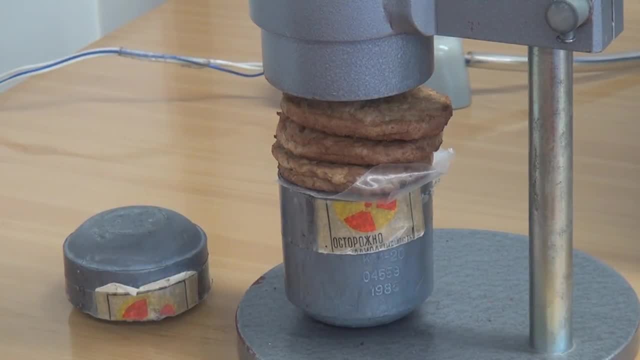 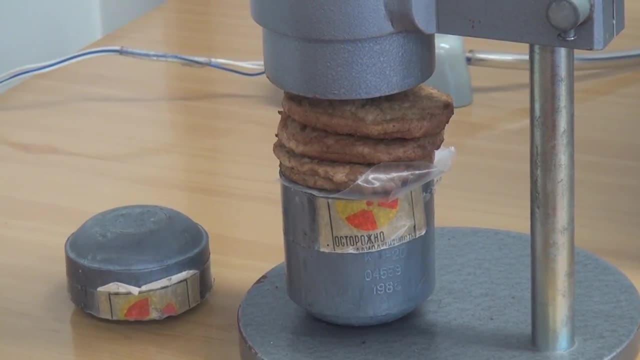 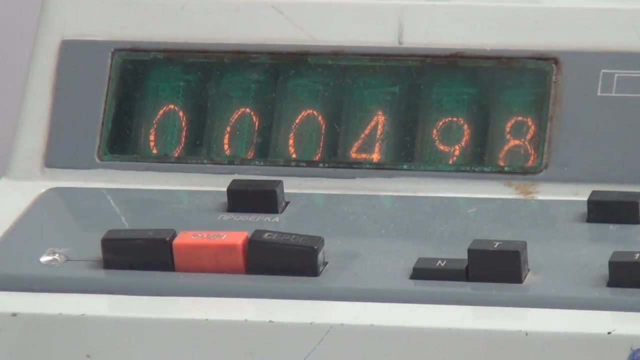 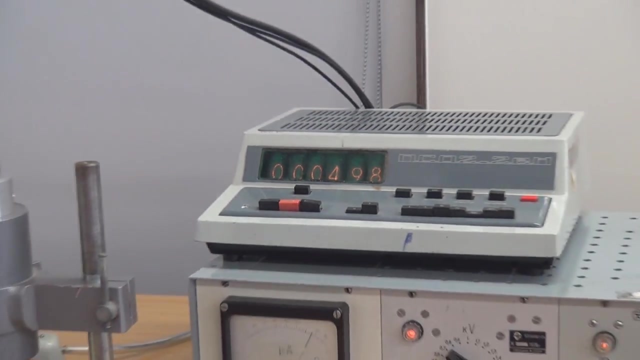 significantly blocked the gamma rays. we tested a bunch of materials, but in an emergency you might think of hiding behind another person in order to get the smaller dose of radiation. so let's test the substance similar to human- a pork cutlet- to see. hiding behind another person would actually help. as you can see, the counter shows 498 counts, which.